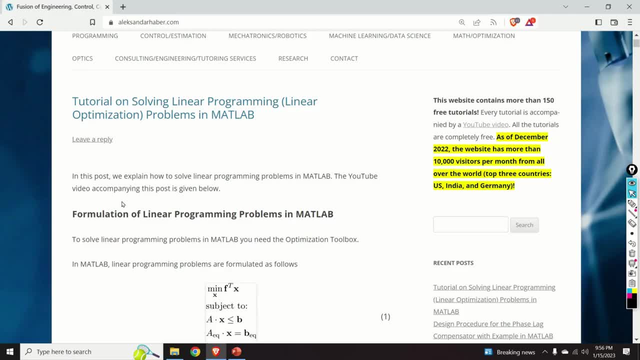 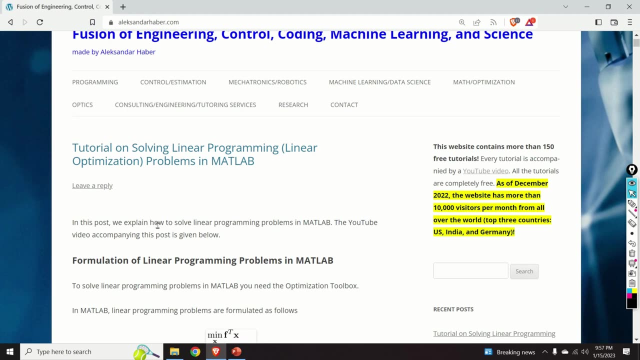 Hello everyone and welcome to MATLAB optimization tutorials. In this tutorial, I will explain you how to solve linear programming or linear optimization problems in MATLAB. Before I start, I would like to mention a few things. First of all, those of you who are my subscribers or who follow my work know by now that I always create a post that nicely. 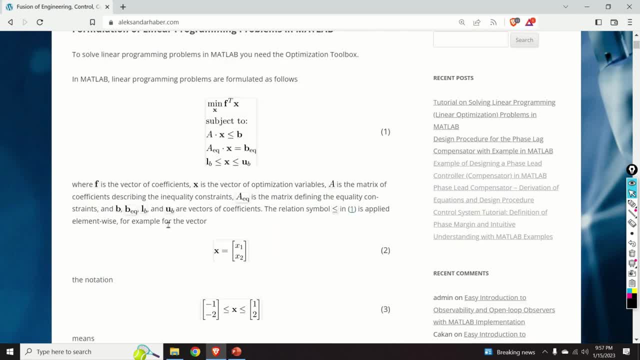 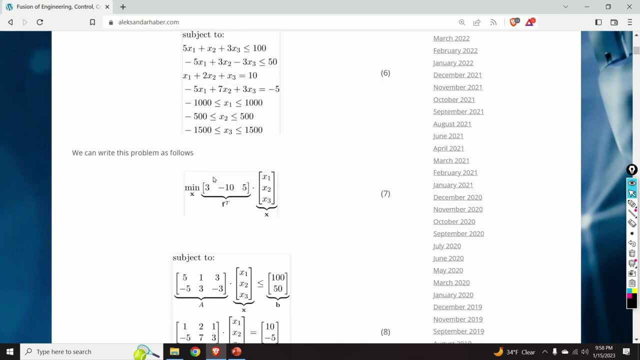 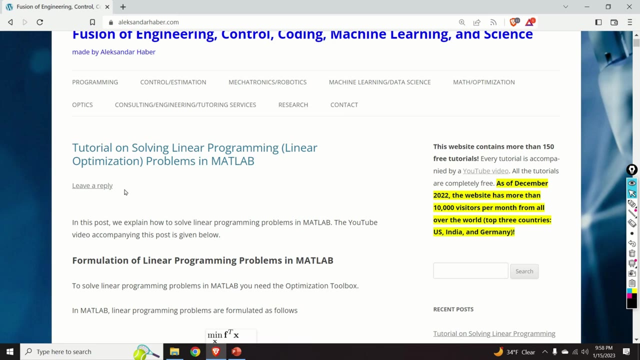 summarizes everything that I will explain in this video And consequently, here is the post. This post contains equations and MATLAB codes. A link to this post is given in the description below. Also, I would like to mention that it took me a significant amount. 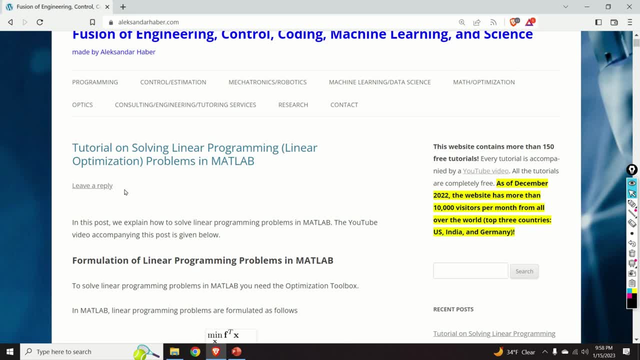 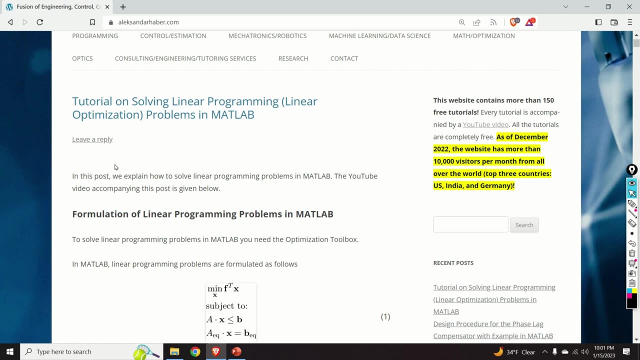 of time, planning and energy to create this video and this tutorial And, consequently, I kindly ask you to press the like and subscribe buttons. Thank you very much. Okay, so let's start. As you will see in this video, under the assumption that you know, 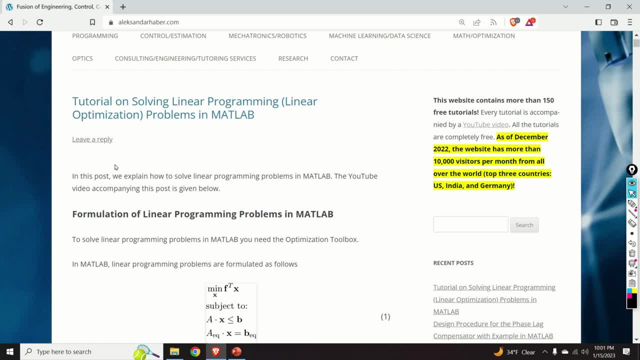 what you are doing. the process of formulating and solving linear programming problems in MATLAB is pretty much straightforward. However, I said under the assumption that you know what you are doing. If you don't know what you are doing, then you might mess up the 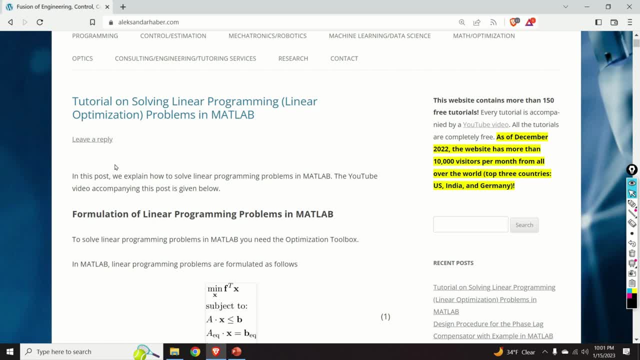 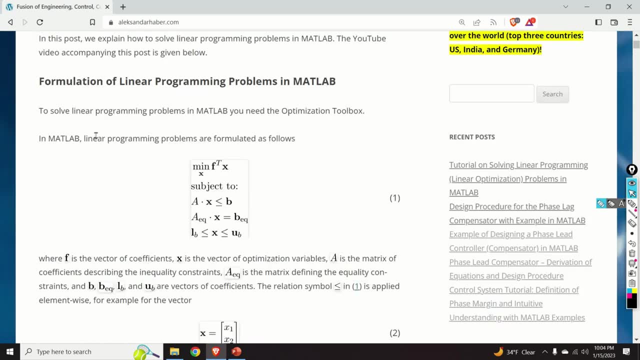 whole solution process and you might not get the most optimal solution Or you might not get the solution at all. Consequently, it is very important to learn the generic form of linear programming problems and how these problems are formulated in MATLAB. The equation 1, given over here, gives a generic form of linear programming problems. This: 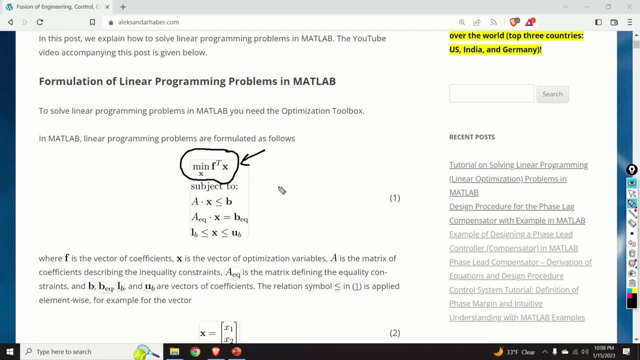 part over here is the cost function. F is a vector of coefficient, The cost function, for instance. X is a vector of optimization variables that we want to determine. On the other hand, this part of equation 1 defines equality and inequality constraints. 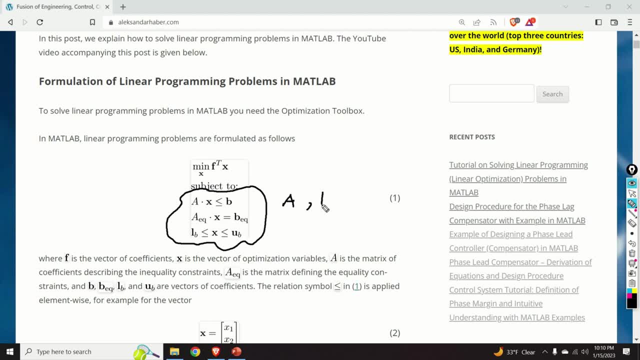 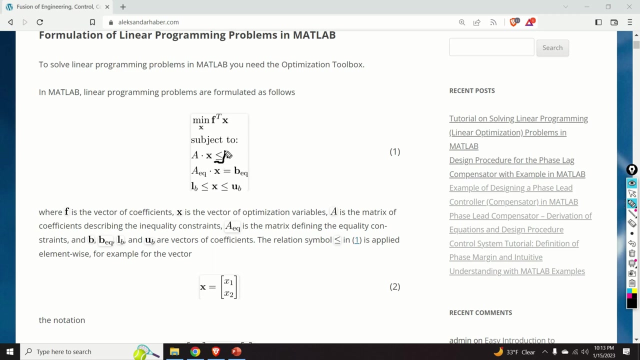 Here, A is a matrix, B is a vector, A E Q is a matrix B, E, Q is grambler And the is a vector, and LB and UB are vectors. Here it's very important to keep in mind that less than or 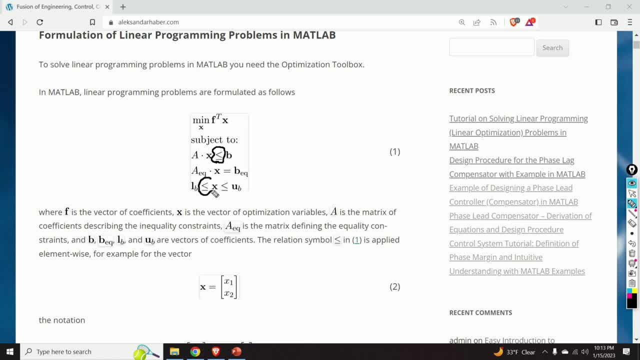 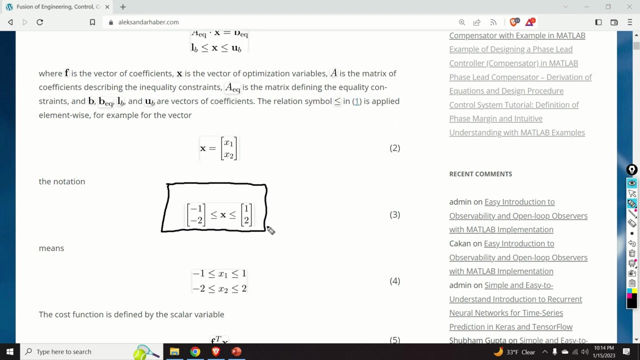 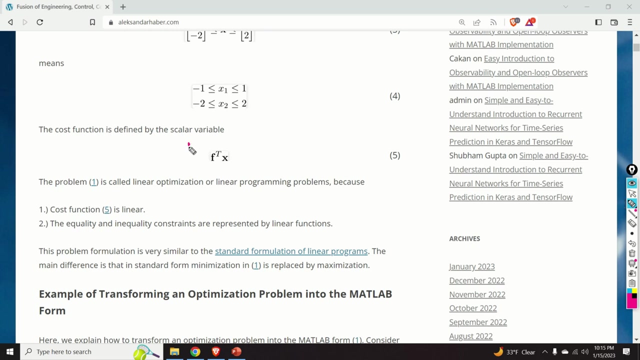 equal to symbol given over here. over here, and over here is applied element wise. To illustrate this, consider the vector X having two variables, X1 and X2.. This notation over here is equivalent to these two inequalities. The cost function is defined by this scalar variable. 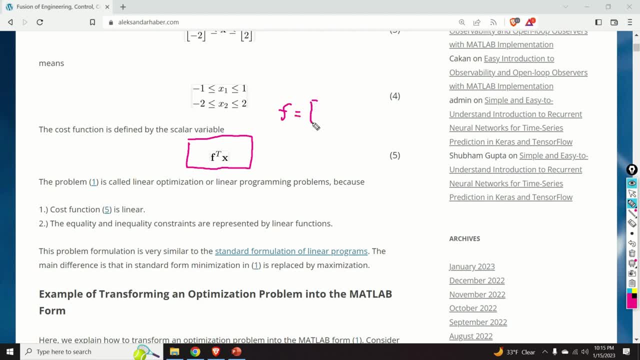 For example, if F is given by F1 and F2 and X is given by X1 and X2, then F transpose times X is equal to F1, F2, X1, X2 and that's equal to F1 times X1 plus F2.. 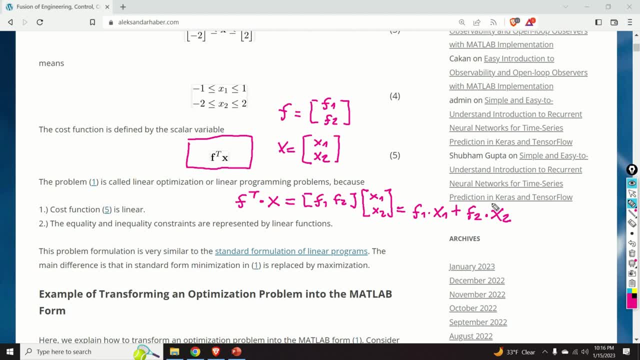 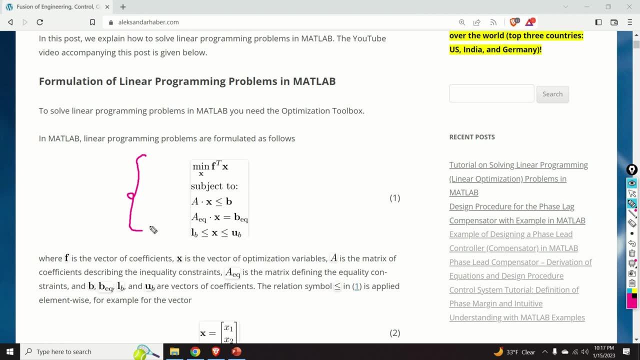 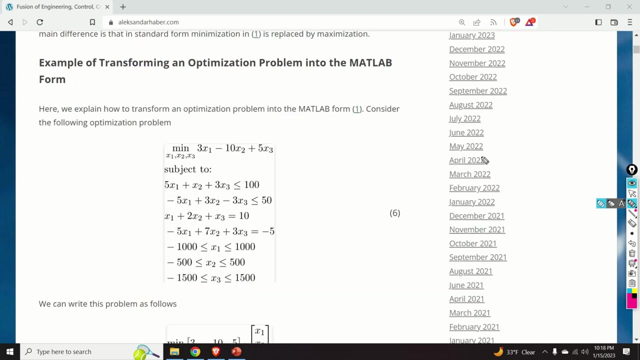 F2 times X2.. The optimization problem given by this equation, that is by equation 1, is a linear program, because number one, the cost function, is a linear function in X and equality and inequality constraints are actually linear functions. Now that we understand the general form of linear programming problems, let us do. 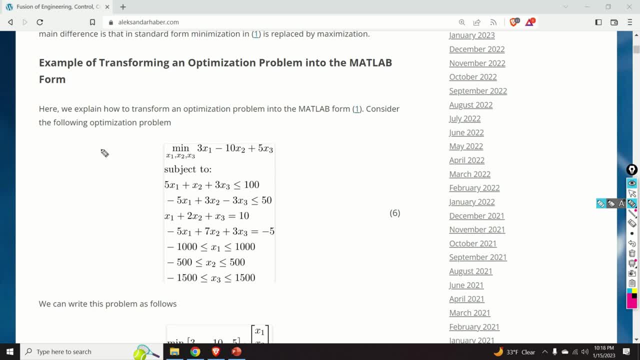 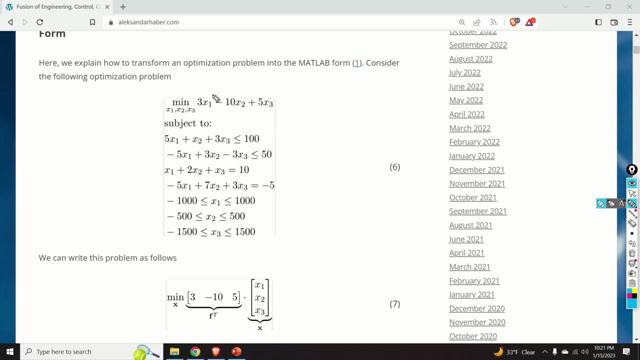 an example. Our example is to transform this optimization problem into the general form. So let's see how to do that. The first step is to transform the cost function into the vector form. Obviously, this is a linear function and I can represent this function in a linear form. 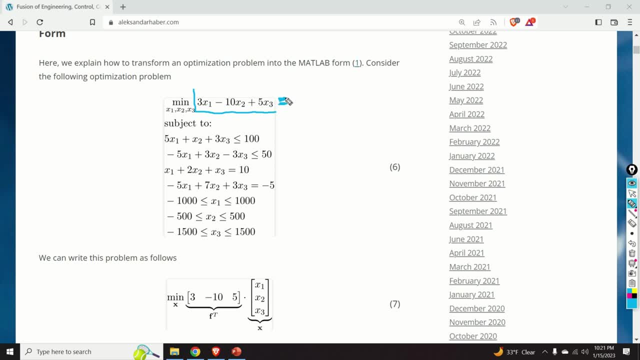 This is a linear function as a scalar product of two vectors. This is the first vector. Its first entry is 3, its second entry is minus 10 and its third entry is 5.. And this is the vector F transposed, and F is accordingly 3 minus 10. 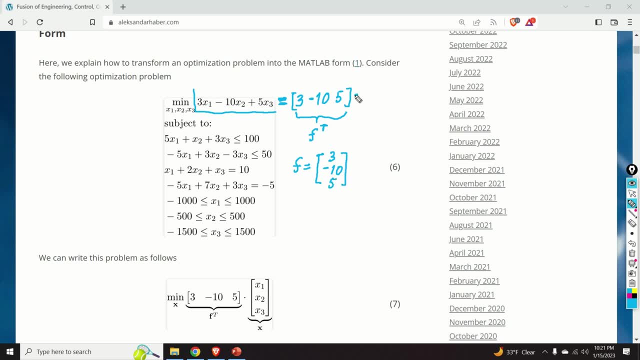 and 5.. Then here I add a dot or scalar product and I need to write the second vector. And the second vector is actually our vector X, whose entries are X1, X2 and X3.. The second step is to transform the constraints. Let us first focus on the 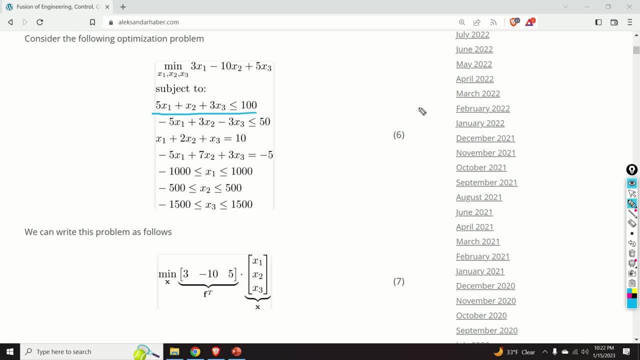 space in this constraint. here, Using a similar procedure, I can represent this constraint as follows: 5, 1, 3 scalar multiplication with X, 1, X, 2, X3, and then I need to add less than or equal symbols. 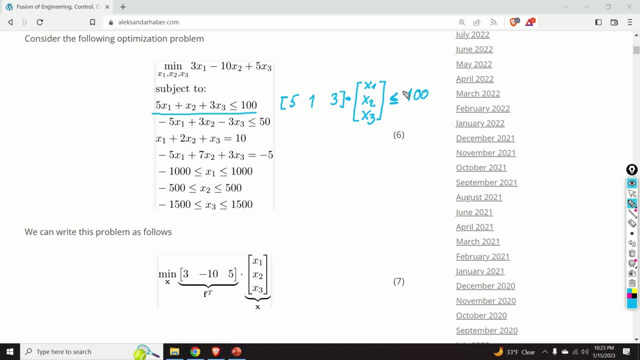 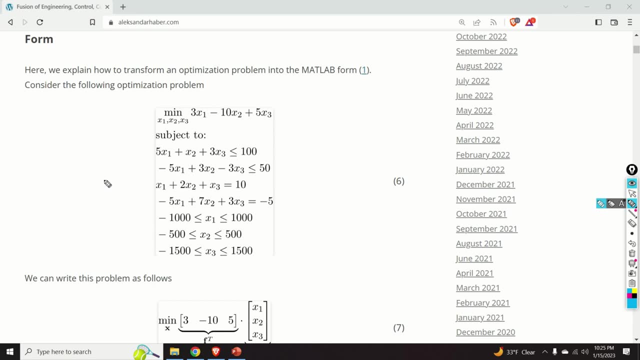 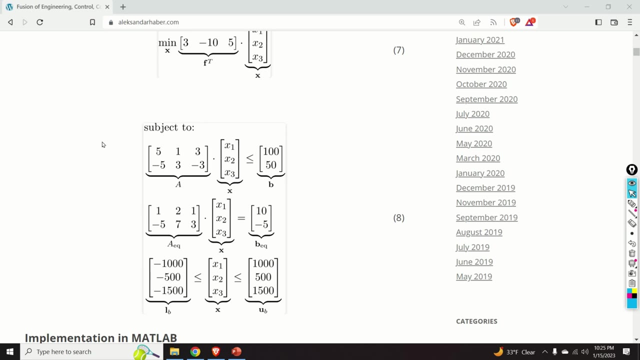 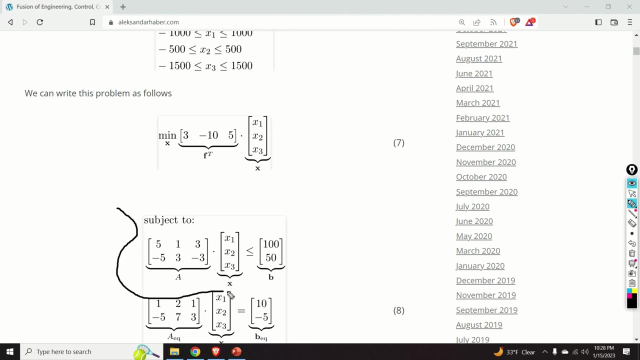 equal symbol and i need to write 100. in the same spirit, we can transform the inequality and equality constraints and, as the result, we obtain a matrix form of equalities and inequalities, and this matrix form is given by the equation number eight. okay, so let us stop here for a second and let us analyze this matrix inequality and let us prove: 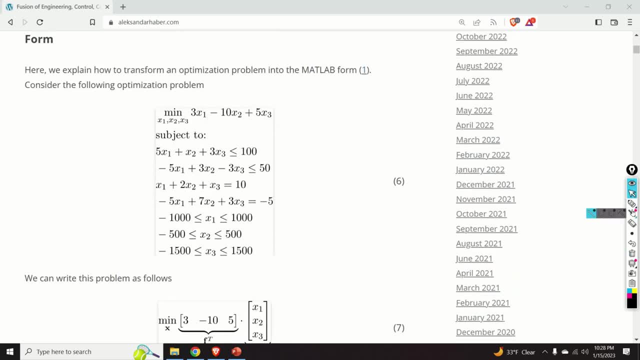 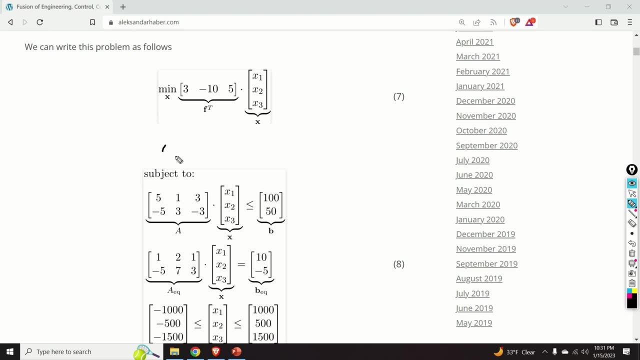 that this matrix inequality is actually equivalent to these two inequalities. to show that we first multiply the first row of the matrix a with a vector x and as the result we obtain x, x minus 5x1 plus x2 plus 3x3, smaller than or equal to 100.. 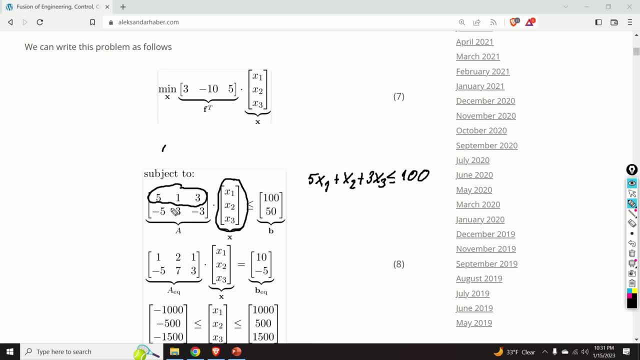 This is the first inequality, And the second inequality is obtained by multiplying the second row of the matrix A by the vector x, And as the result we obtain minus 5x1, plus 3x2, minus 3x3 smaller than or equal to 50.. 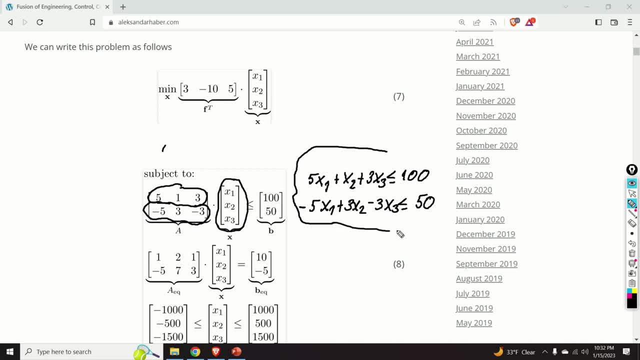 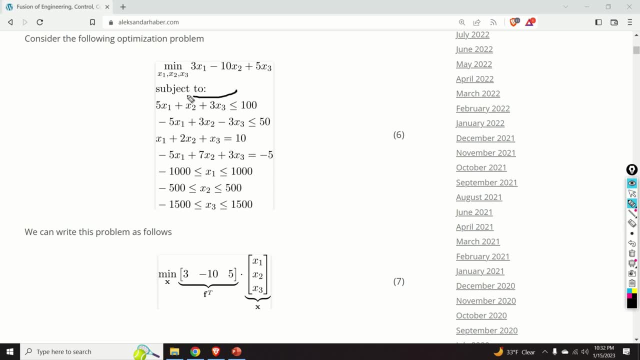 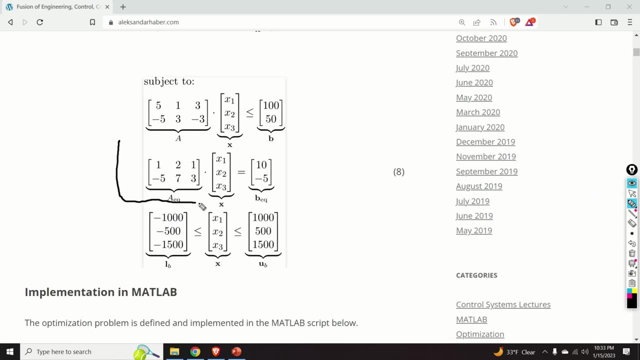 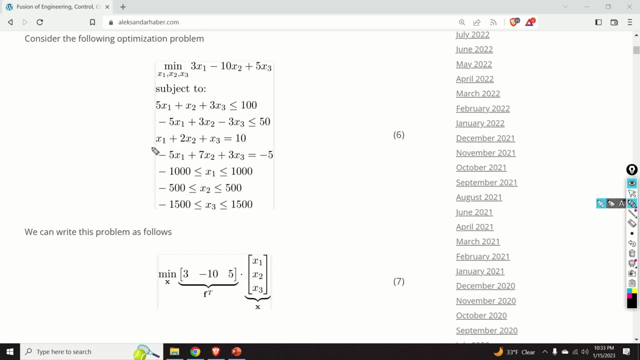 Obviously, these two inequalities are precisely the inequalities given in our original optimization problem. Similarly, you can show that this matrix A, this equality, or better to say matrix equation, and this vector equation are identical, or better to say, equivalent to the original equalities. 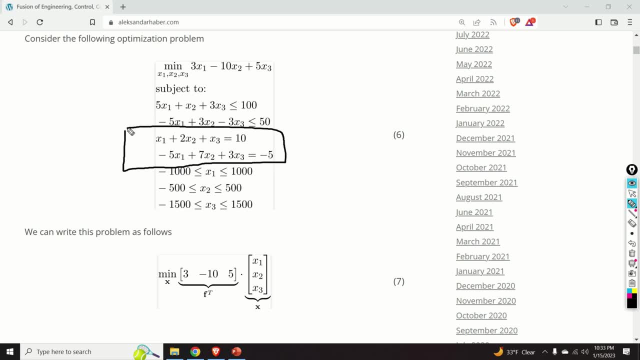 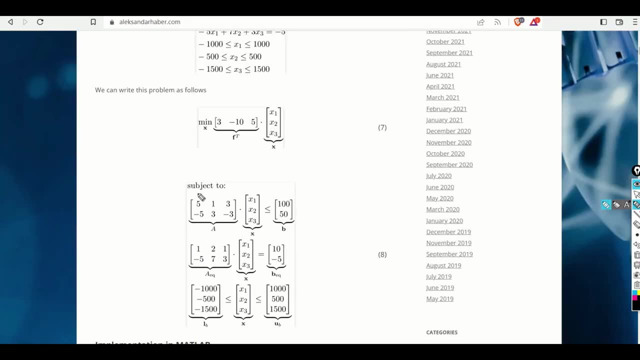 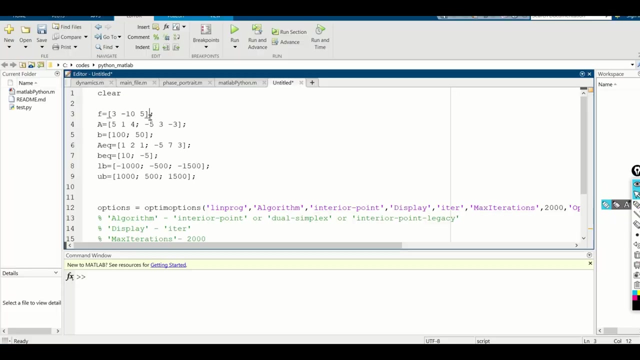 given by these two equations and by these inequalities. From this vector and matrix formulation of the optimization problem, we can directly read: the vector F, matrix A, vector B, matrix, veq, lower-bound and upper-bound vectors. Next, let us learn how to implement this optimization problem in MATLAB. 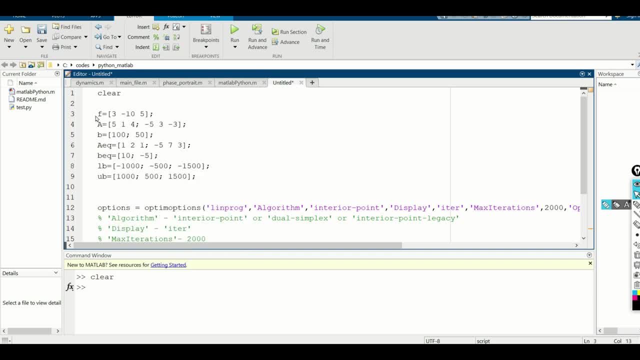 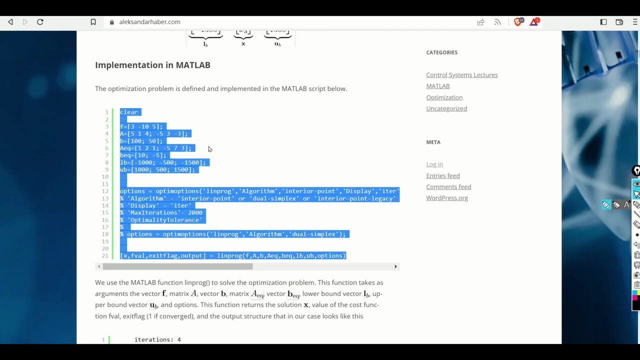 First I will clear my workspace. Then I will simply define my vector A, matrix A, vector B, AEQ, BEQ and the vectors lower bound and upper bound, As I mentioned previously. you can simply read these values from this problem formulation. Let: 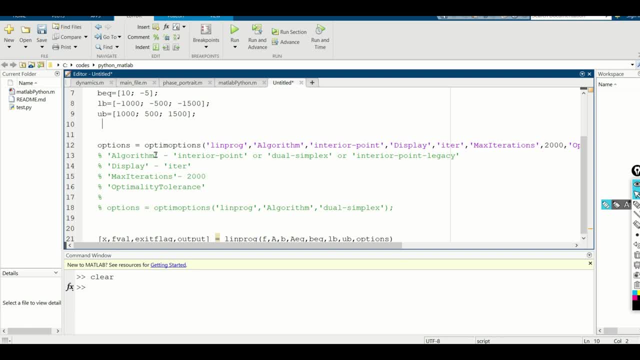 us go back to our MATLAB. Then the next step is to define the optimization options. In this case, I will be using linprog MATLAB function. Then I need to define my algorithm. The algorithm will be interior point algorithm. During the solution process, I want to display iteration progress. Consequently, I 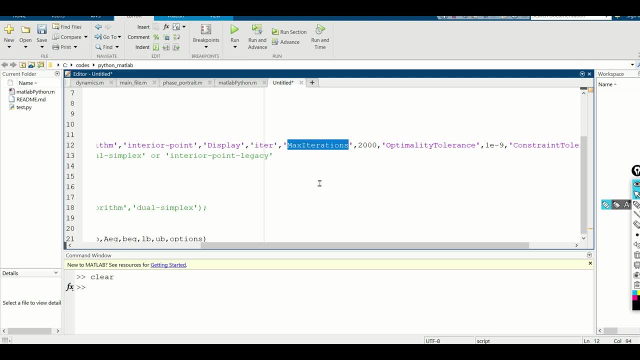 specify this parameter over here. I specify the max number of iterations- I don't want to go above 2000 iterations. Then I specify the optimality tolerance, that's 10 to the minus 9, and I specify the constraint tolerance. The constraint tolerance is 10 to the minus 6.. Here you can use other solvers. 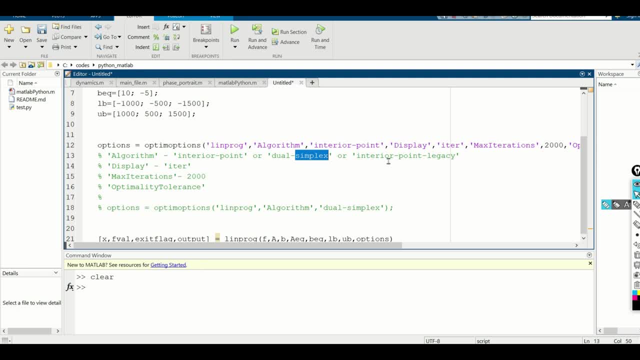 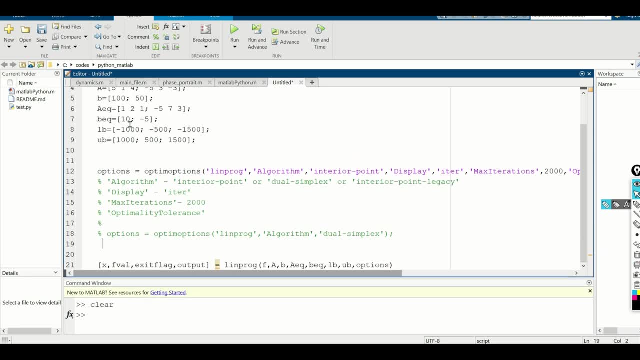 For example, you can use dual simplex or interior point legacy. Finally, once we defined the matrices and vectors and specify the options, we simply call this function linprog. We specify the vectors and matrices: lower bound and upper bound. we specify the structure Defining the optimization. Specify the optimization: solvers: parameters. 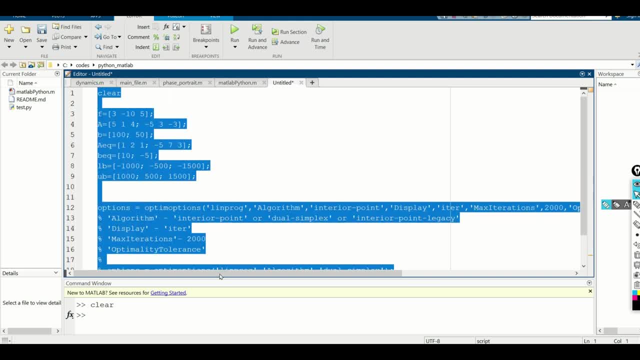 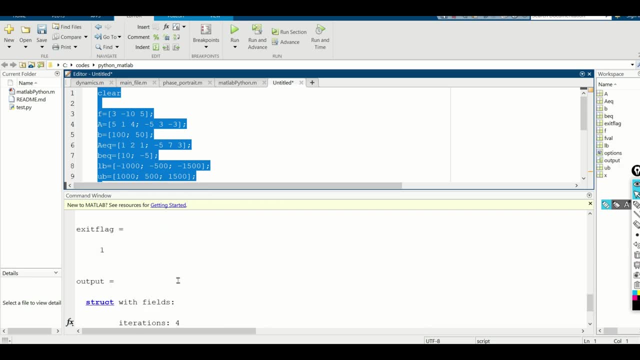 Let us execute this code. Let us see the result. Here I will expand the command window. and let's evaluate the meal section. Here we have the solution. The X is our solution. This is the value of the cost function. The exit flag means that we have actually solved the problem. 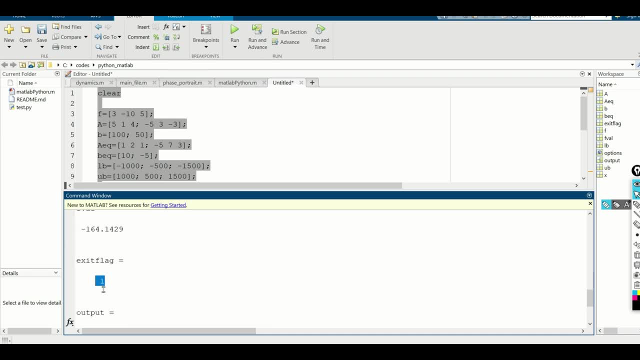 This means that we are back to actually solving the problem problem If you obtain zero or some other value, it means that you didn't successfully solve the problem and you have an output giving you more information about the solution process. We are using an interior point method, and these are some parameters that I will not explain in this video. 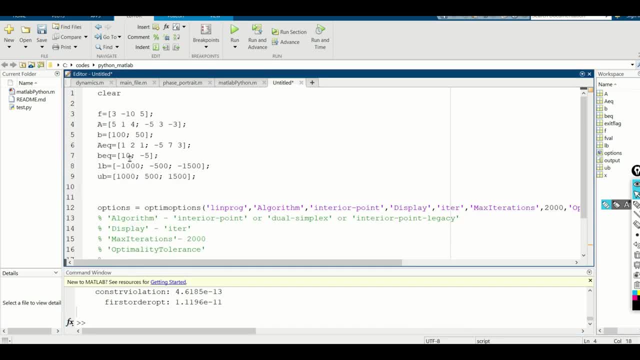 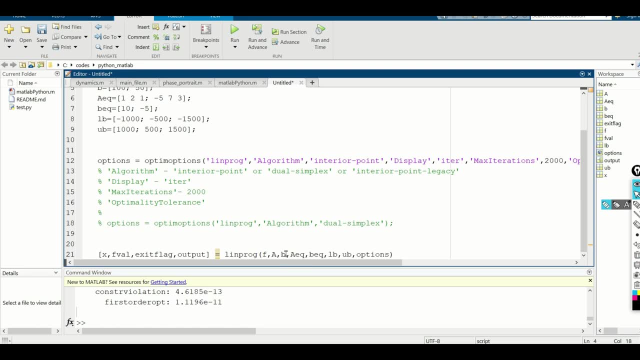 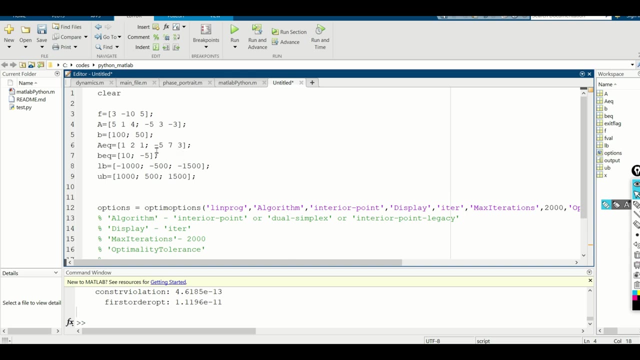 In some optimization problems, we might not have equality or inequality constraints, and the question is how to eliminate some of the equality or inequality constraints from this problem formulation and from our solver, and the solution is pretty much straightforward. For example, if you want to eliminate the equality or inequality constraints, you will simply define them. 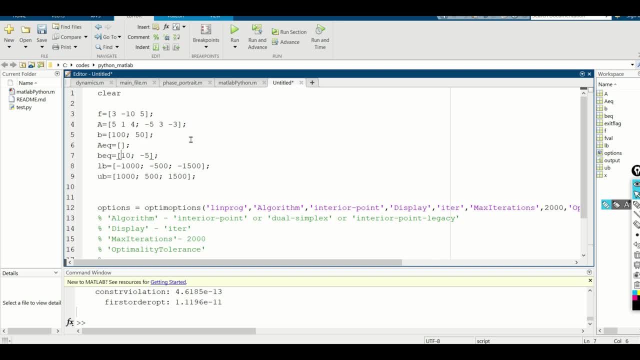 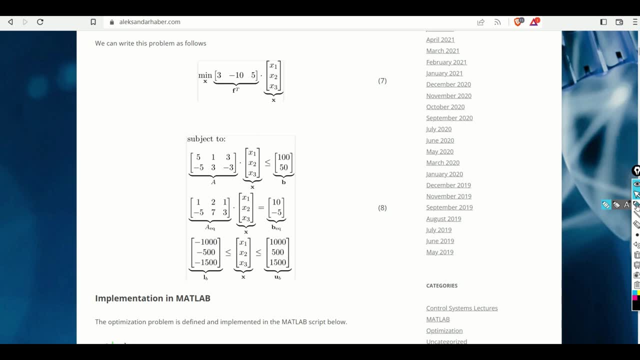 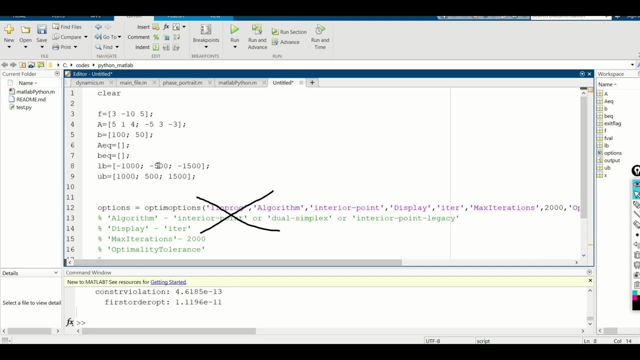 as empty matrices. So here we will specify an empty matrix and here we will specify an empty matrix. This means that we actually don't have a equality constraints. So, going back to our MATLAB code, we can simply rerun the code with these parameters and let's see the result. 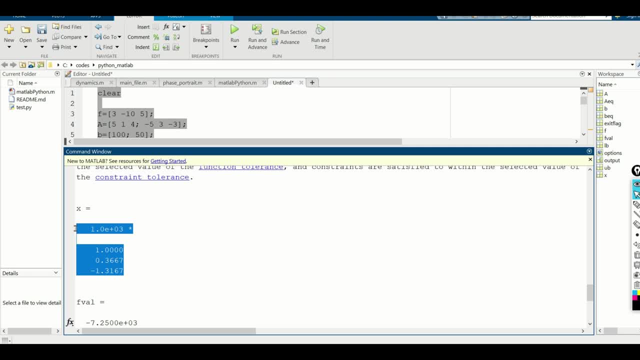 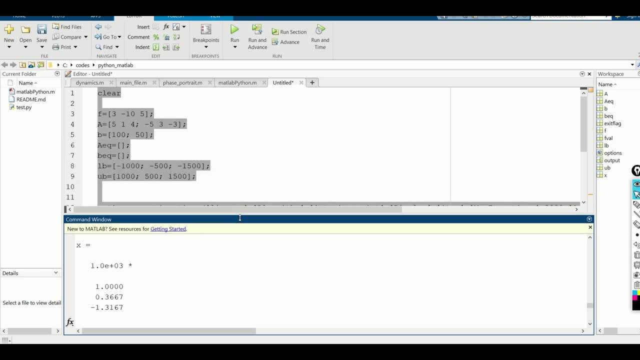 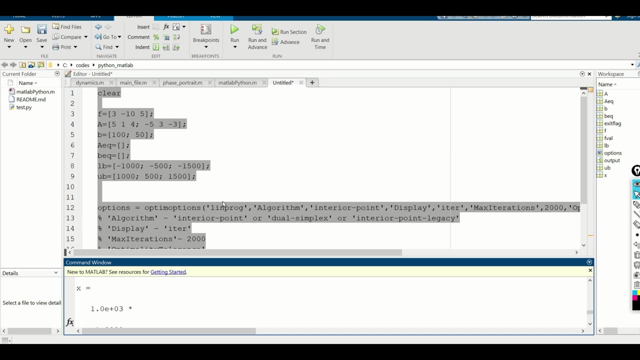 And here's the solution. and obviously the solution is quite different and the value of cost function is, of course, much smaller, since our problem is less constrained. Okay, that would be all for today. I hope that you like this video. If you like the videos I create, please press the like and. 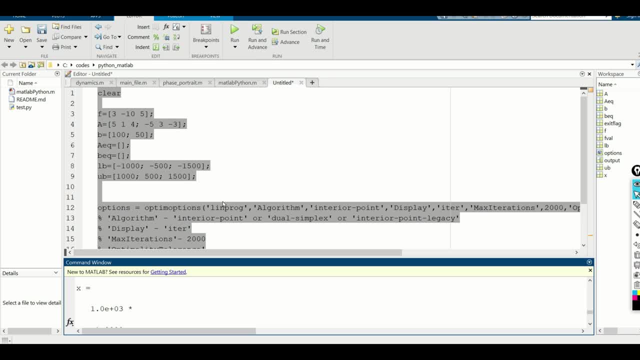 subscribe buttons or even consider to support my channel. Thank you very much and have a nice day.